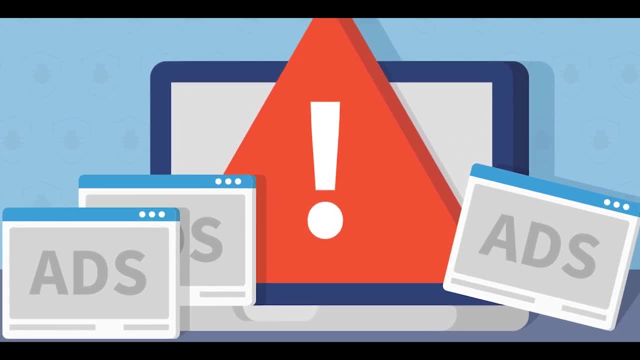 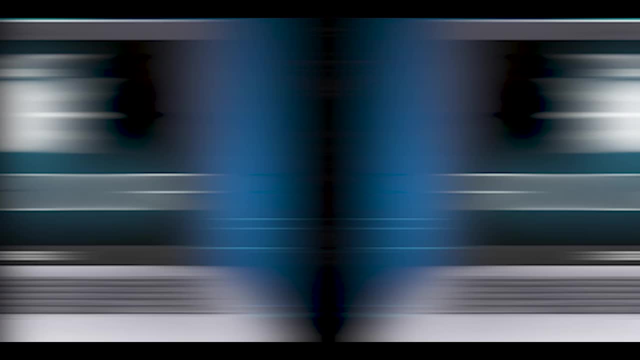 advertisements in the interface of the software or on a screen presented to the user during the installation process. Next, we have a backdoor, and backdoor refers to any method by which authorized and unauthorized users are able to get around normal security measures and its specific safety measures. 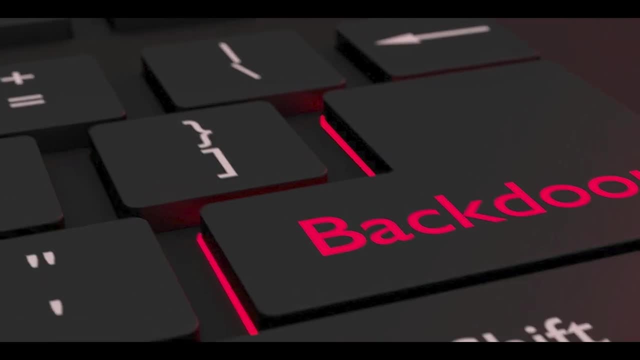 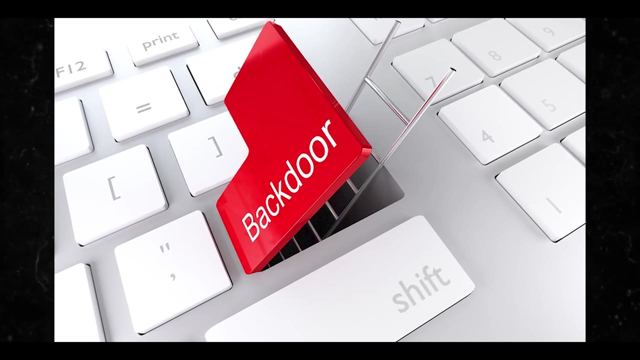 In addition, the method influences users' interaction with touchリne social 1994.. source crashes, Willy VO, etc. measures and gain high level access, user access, aka root access on a computer system, network or software application. uh so uh, before i proceed, please take a moment to hit the subscribe button. 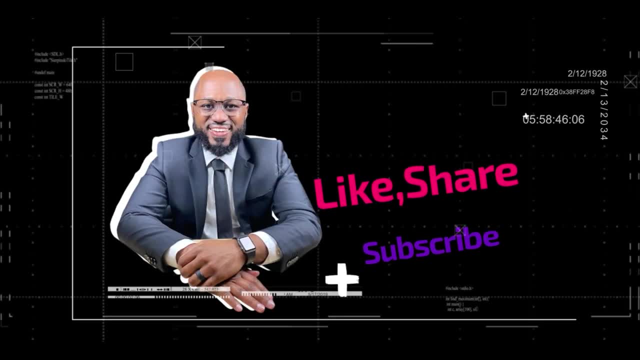 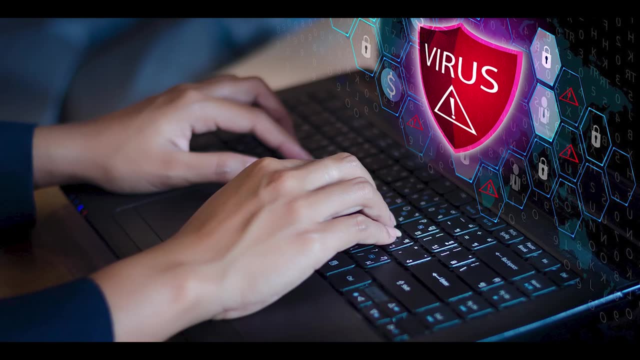 and the like button. please take a moment to hit the subscribe button and the like button. next we have a computer virus, which is a type of malware: when executed, replicates itself by modifying other computer programs and inserting its own code into those programs. next we have a. 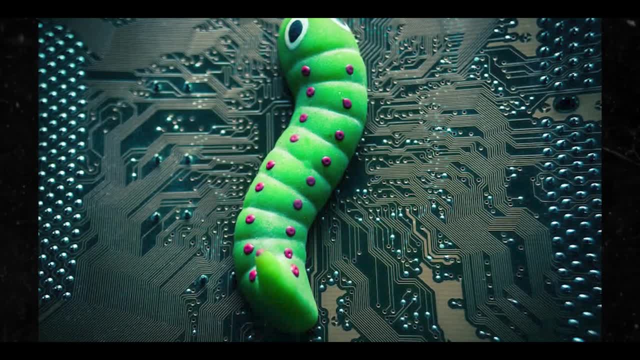 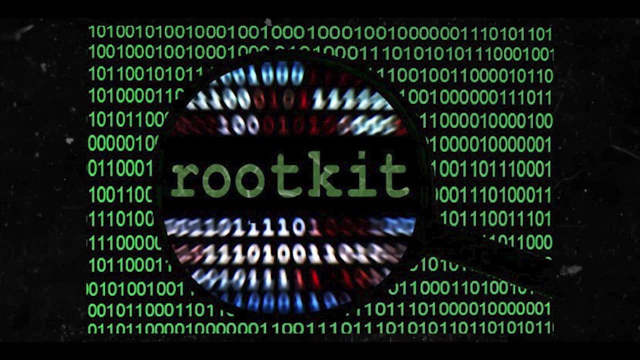 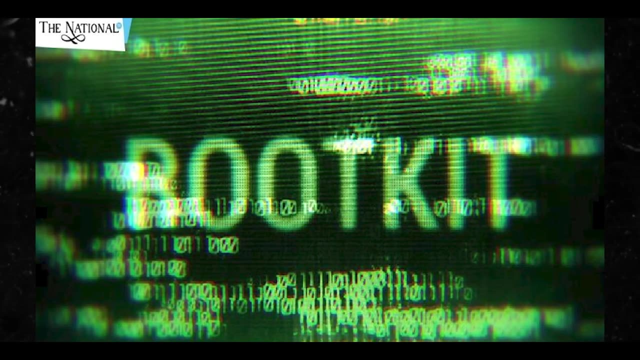 worm. a computer worm is a standalone malware computer program that replicates itself in order to spread to other computers. uh next we have rootkit, and rootkit is a software used by cyber criminals to gain control over a target computer or network. uh next we have crypto jacking and 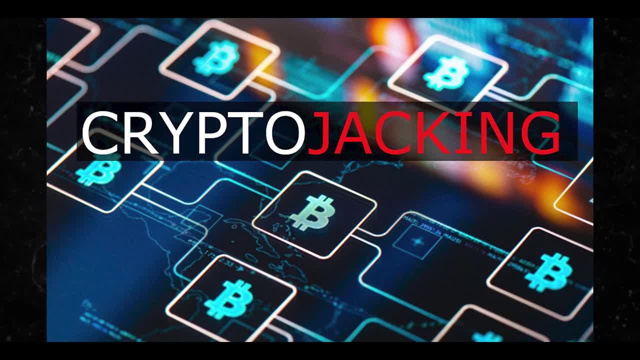 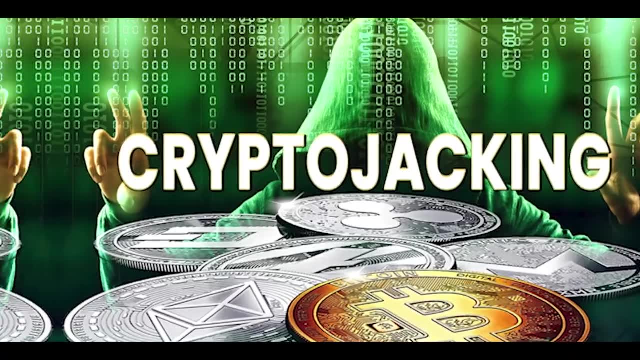 crypto jacking is the act of exploiting a computer to mine cryptocurrencies, often through websites, against the user's will or while the user is unaware. uh, next we have phishing, and phishing is a form of hacking, and phishing is a form of hacking, and phishing is a form of hacking. 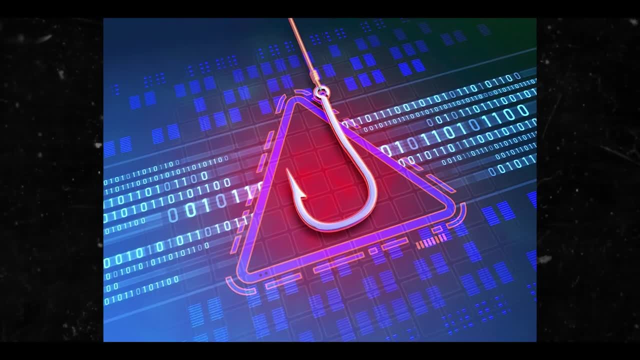 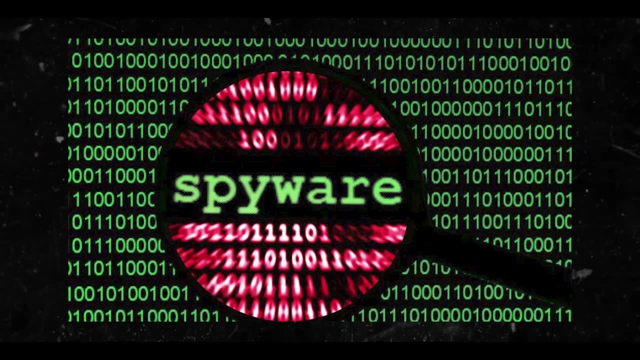 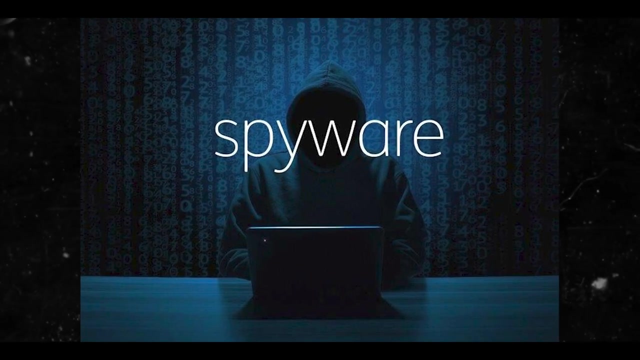 of social engineering and scam, where attackers deceive people into revealing sensitive information or installing malware such as ransomware. next we have spyware, which is any software with malicious behavior that aims to gather information about a person or organization and send it to another entity in a way that harms the user by violating their privacy. 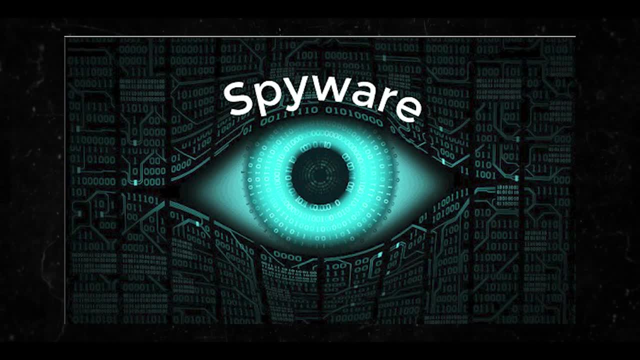 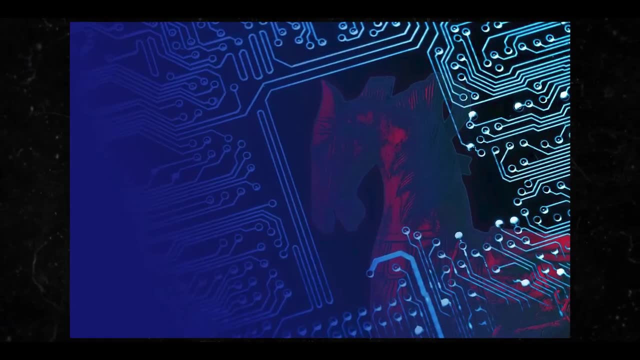 endangering their device's security or other means. next we have trojan horse, and that is any malware that misleads users of its true intent by disguising itself as a standard program. uh, next we have a wiper, which is a malware that deletes or destroys any organization's access to. 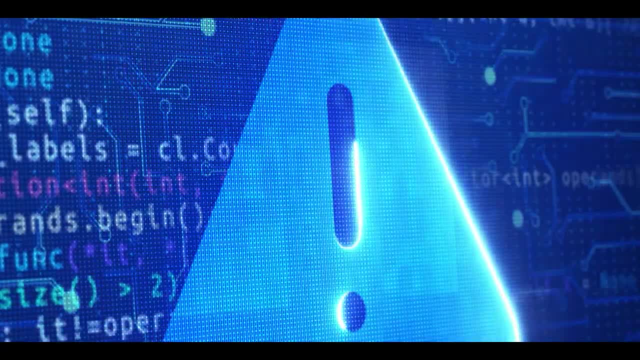 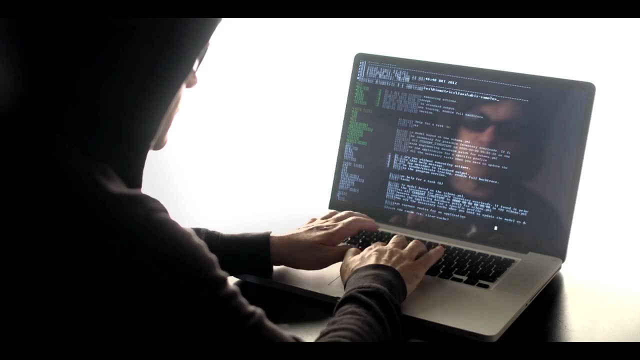 files and data, the. this file is a malware that is commonly used as a tool for destruction and disruption, since the loss of critical information could make it impossible for an organization to maintain business operations or carry out certain actions. uh, next we have keylogger, and that is. 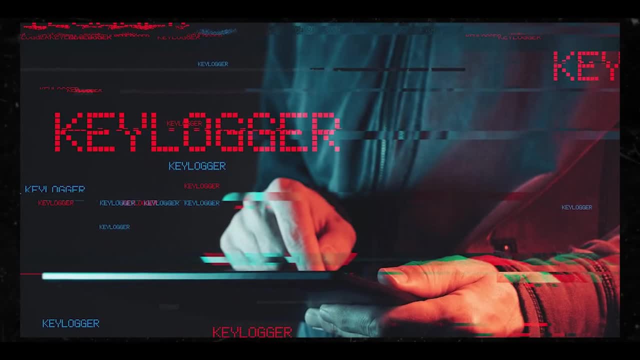 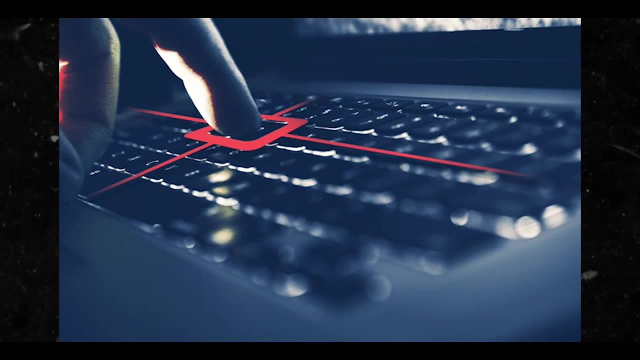 often referred to as keylogging or keyboard capture, which is the action of recording the key struck on a keyboard, typically called a keylogger, and that is often referred to as a keylogger covertly, so that a person using a you know the keyboard is unaware that their actions are being.